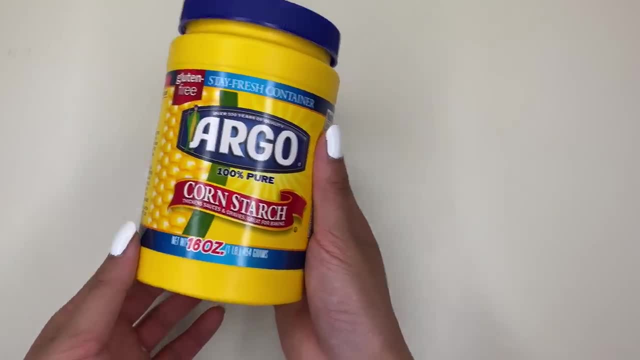 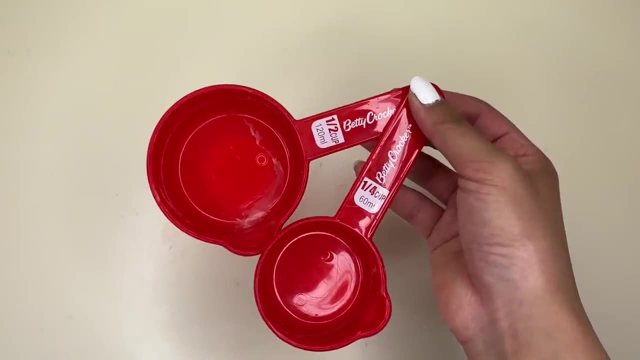 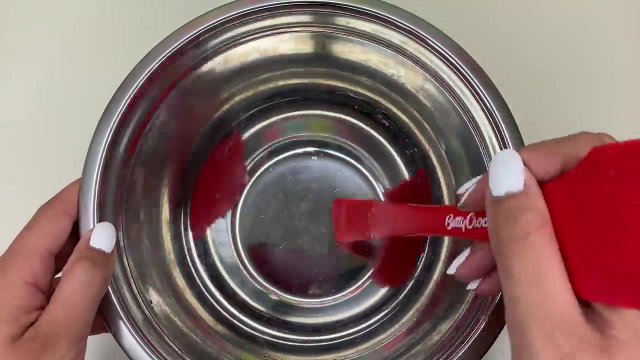 need any type of hair conditioner, cornstarch, food coloring and a half cup measuring cup and a quarter cup measuring cup. You can really use any size measuring cups because it is a one to two ratio, But I'm just using these today to make it easier. A mixing bowl and any mixing utensil of. 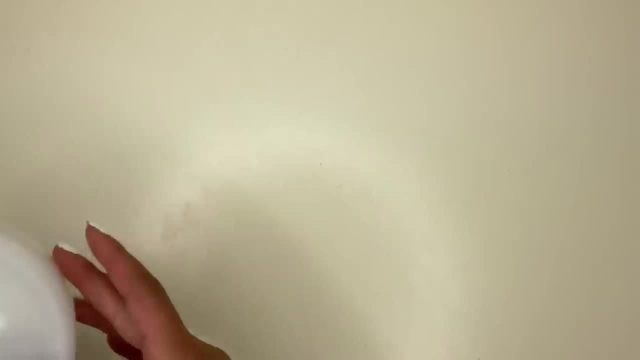 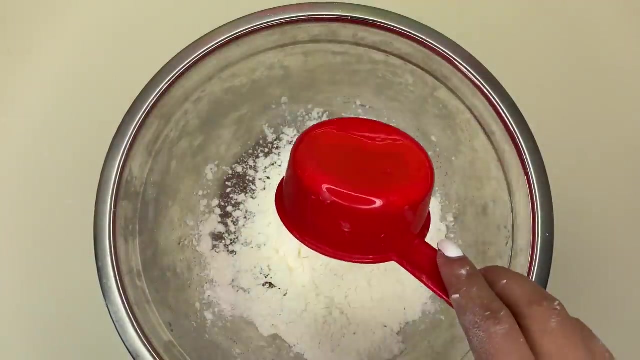 your choice And some airtight containers. All right, so let's just get right into this. Um, no mess, Sure. So now you're going to add in a half a cup of cornstarch, a quarter cup of hair conditioner. As I mentioned earlier, this is a one to two ratio, So one part. 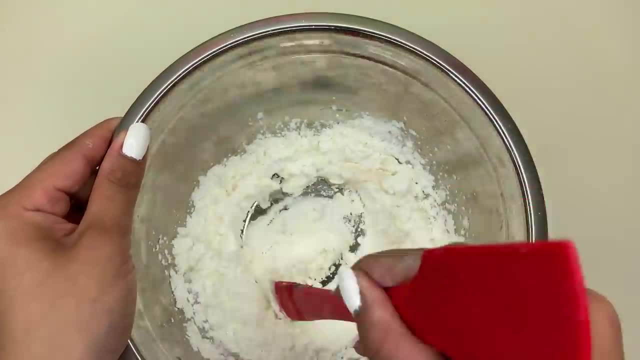 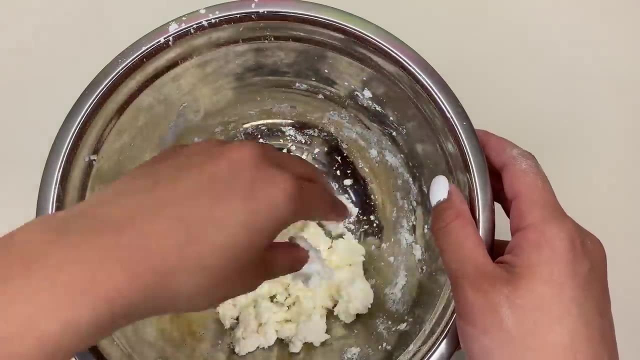 conditioner and two parts cornstarch, So you can really alter this recipe to make however much you want. Now you're just going to mix it all together, So it should start to clump together and give you this gross like expired cottage cheese texture, And then you can go in and start kneading it with. 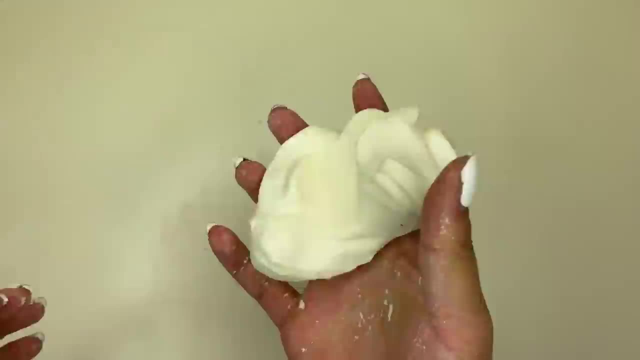 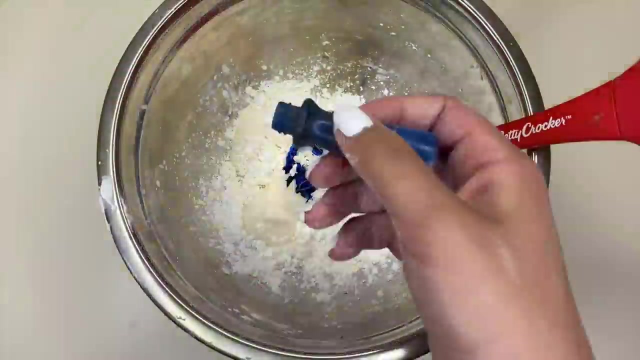 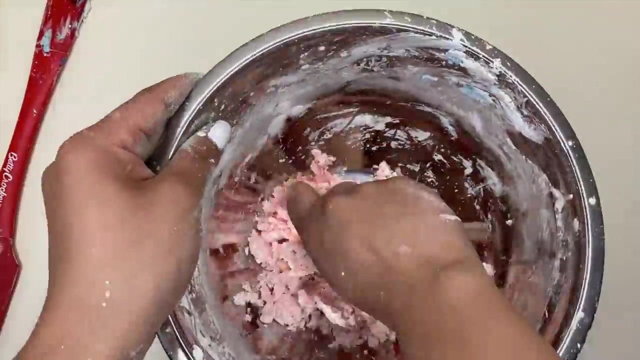 your hands. if you feel comfortable, It should start clumping together and then create this awesome looking clay. This whole process literally took me a matter of maybe like five minutes to do, So I'm just going to take a container and make some blue, green, red or pink and yellow therapy. 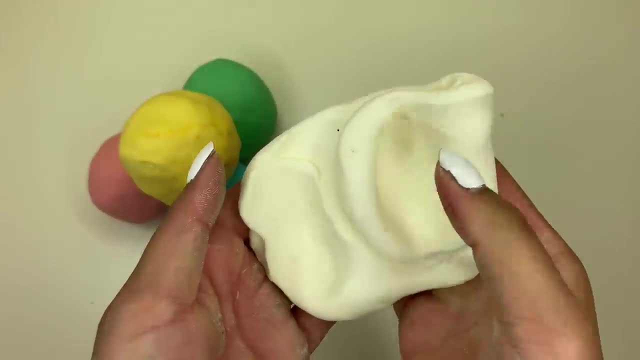 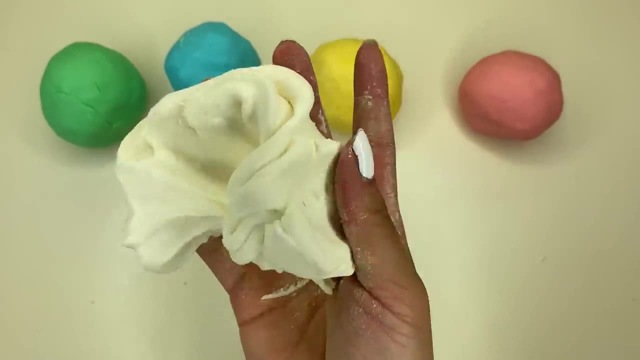 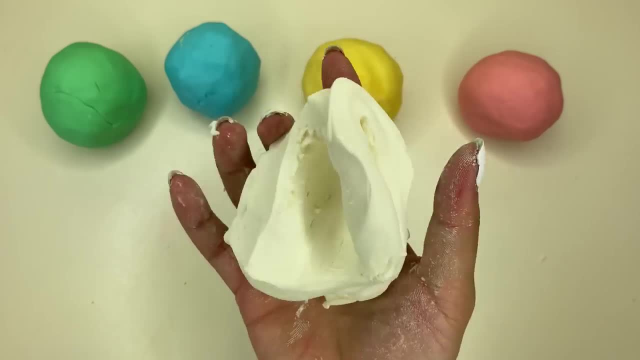 going to go ahead and mix it all together. So I'm just going to go ahead and mix it all together. So cornstarch is one of the main components in it. It doesn't really have a long shelf life. I would literally give it like a couple hours before it starts to get all dried out and crusty I mean. 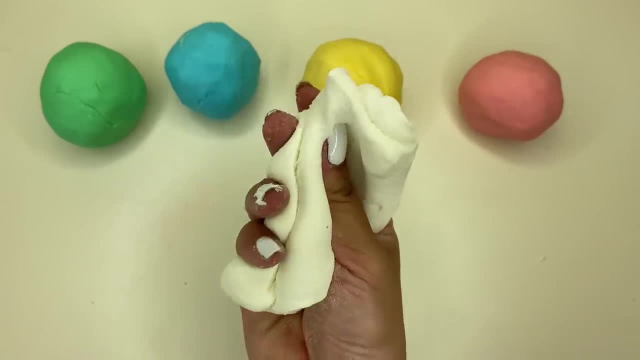 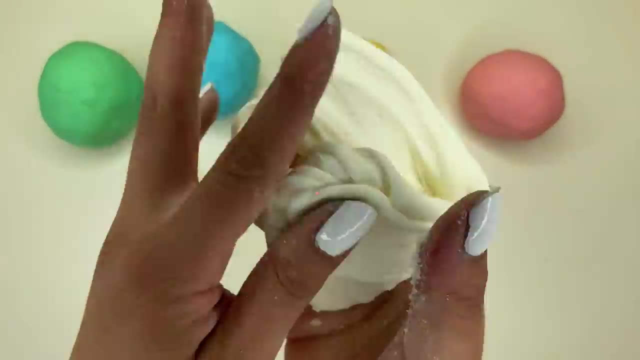 just with these little balls sitting there for a matter of five minutes for me to film this ASMR, they already started to get dry and cracked out. I mean, I'm sure you can soften this with some water or more hair conditioner, but the maintenance just really isn't worth the experience for me. 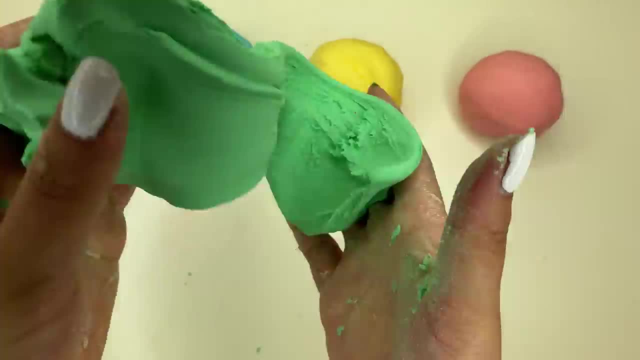 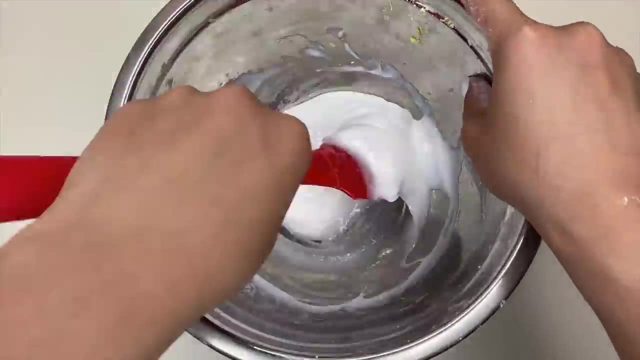 But for how cheap, simple and quick this is to whip up in your free time, I would definitely say that this is a notable recipe. All right, So I'm going to save you a lot of blood, sweat and tears and mess, because I was feeling like a little bit of Bill Nye, the science guy, today And I wanted 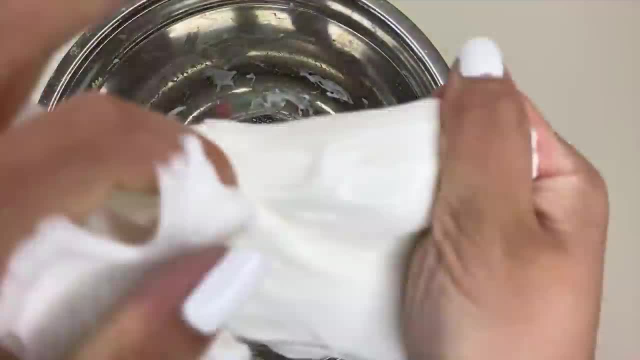 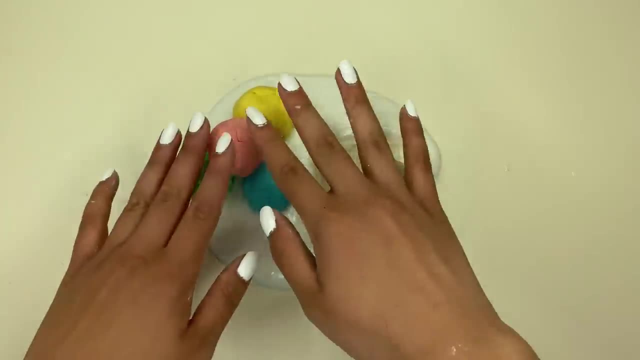 to see if this clay would make a butter slime out of a regular slime. So typically, to make a butter slime you would add clay to a regular school glue based slime and it would thicken it up and give it a creamy and soft texture. Well, no, not with this one. It completely melted the slime. So I guess 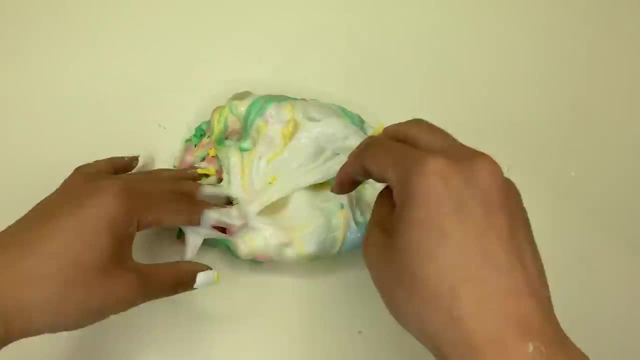 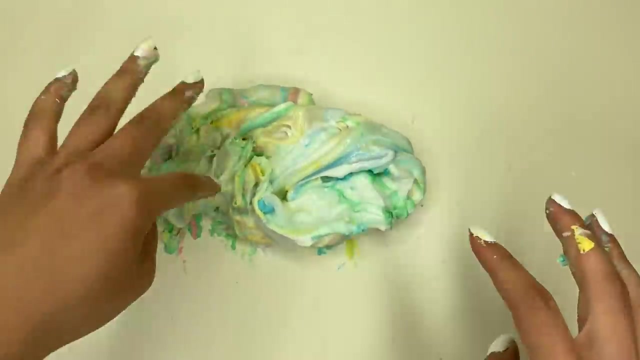 if you want a slime softener, this is your go to, But do not add this into slime, Just don't do it. So I'm going to have the ASMR of this mess and the little clay balls at the end of this video. 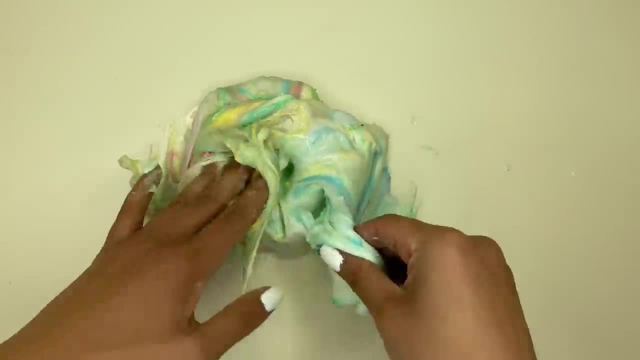 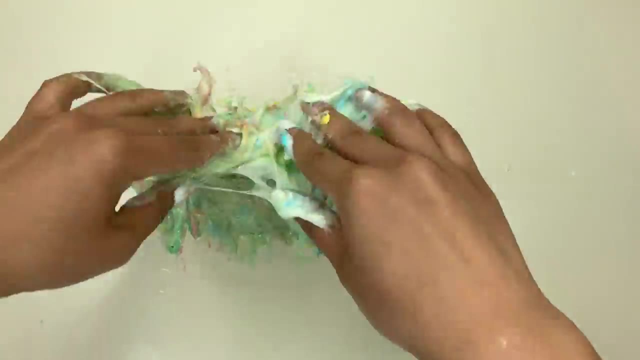 But I just wanted to come in here and say I hope you guys enjoyed this video. I'm sorry that it is shorter than most of my videos. I honestly forgot how short my tutorials are, but I feel really guilty for jipping you guys off from content. 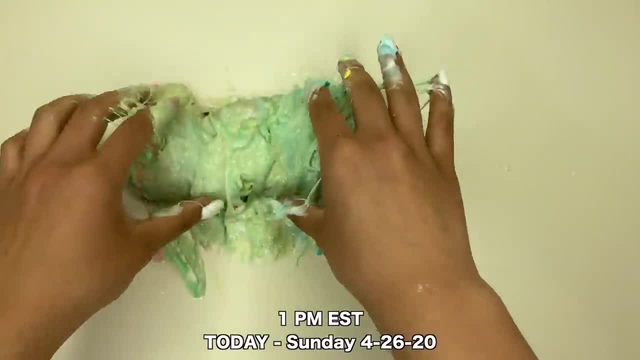 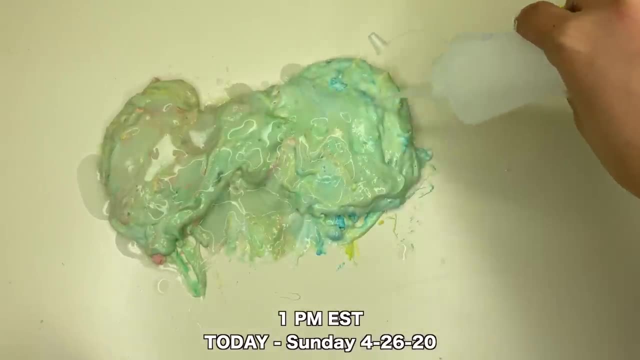 So I'm going to be going live at 1 pm Eastern Standard Time for an hour where you guys can ask me all of your questions. So I haven't gone live in a long time and I'm actually really excited to do that. So I'll be sure to see you guys there. So I really hope you guys enjoyed this video. If 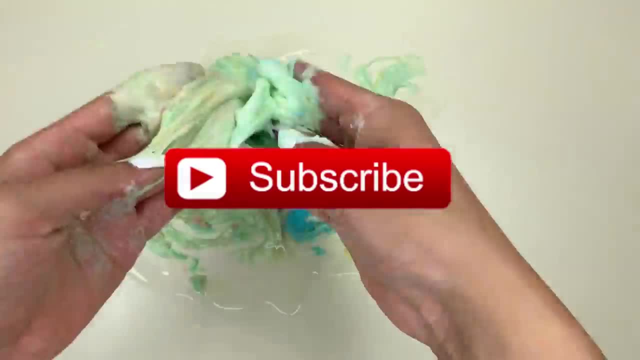 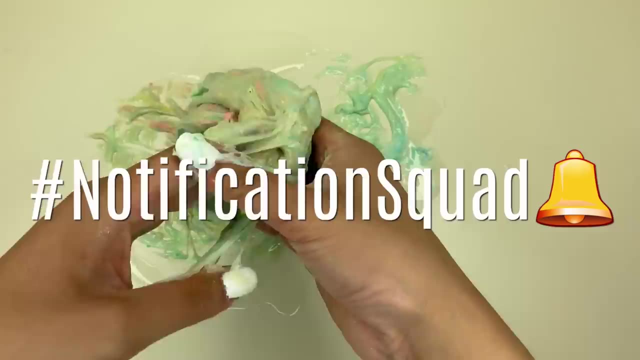 you did make sure to give it a big thumbs up and to hit that big red subscribe button down below and the little post notification bell right next to it to get notified every time I post a new video. By doing this, you'll become a member of the hashtag notification squad and one of my timers. 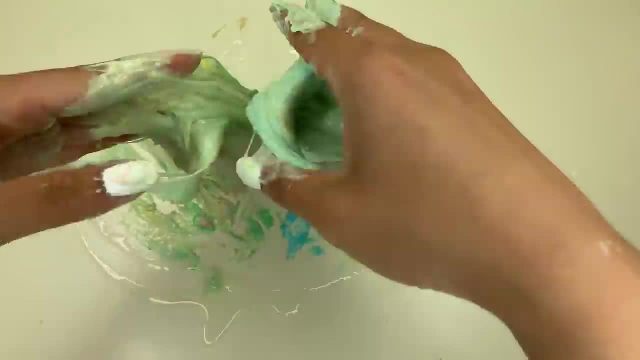 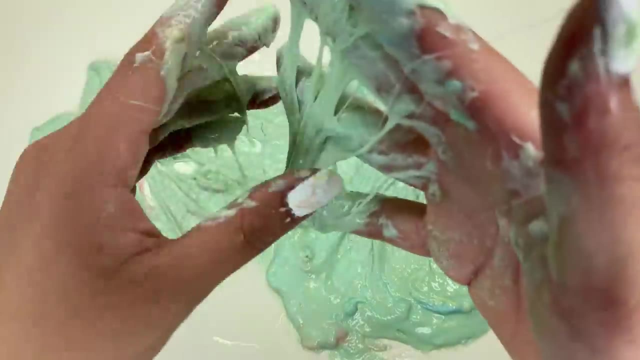 So I'll see you guys in the next video. Bye, Oh, I'm just watching this video right now And this mess is literally giving me like PTSD. That was one of the worst messes I've had to clean up in a while, So I'm just going to stop rambling.